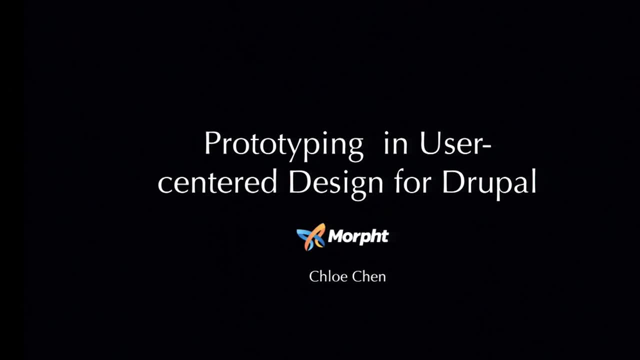 Hi everyone. I'm going to talk about prototyping in user-centred design for Drupal today. A bit about myself: My name is Chloe. I'm a UX designer and front-end developer at Morphed. I started interactive multimedia system design at UTS and have been working with Drupal for the past. 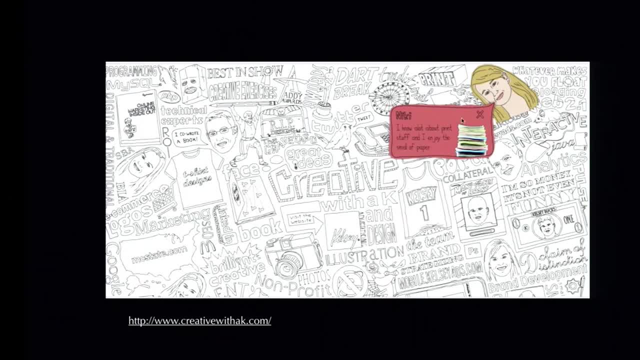 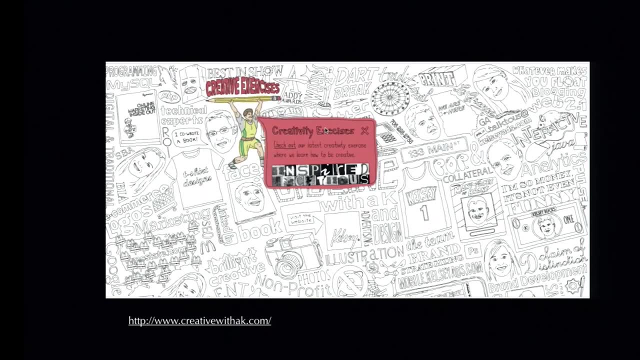 two years. I ran into this website the other day. Can anyone tell me what's wrong with this website? Anything else, I mean? what's the problem with this website Exactly? As a user, I struggle to use it. It's fancy, It's artsy, It's creative, It's totally out. 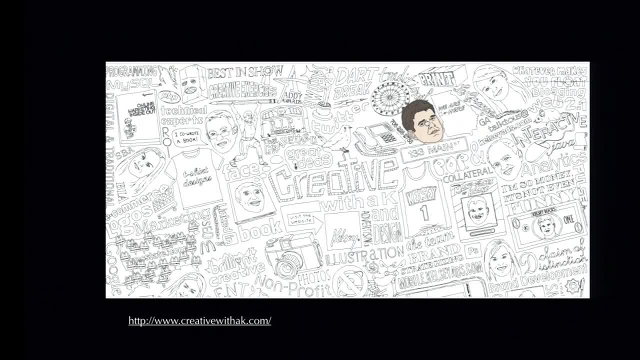 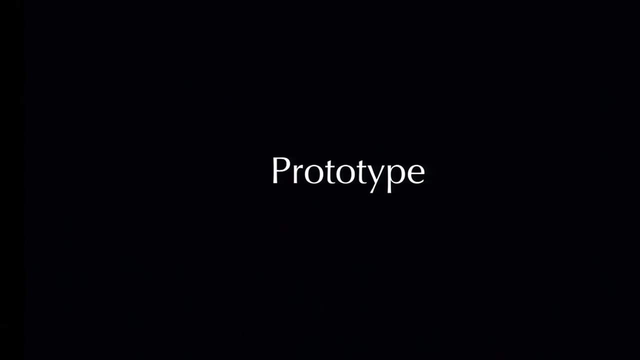 of the box, But as a user, I find big usability problem with it. There are plenty of websites out there that has the similar issue. It looks nice, It's so creative, But it's not for the users. So my topic today is: 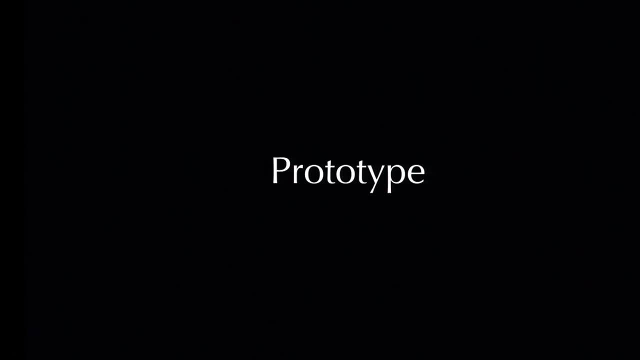 I'm going to talk about this, one simple thing we can do to avoid usability problems. First of all, I like to define what prototype is and isn't, And then I'm going to talk about different prototypes and different tools we can use to create them. And finally, I'm going to talk about usability. 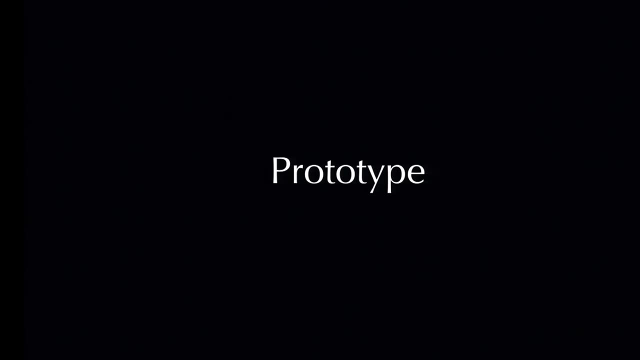 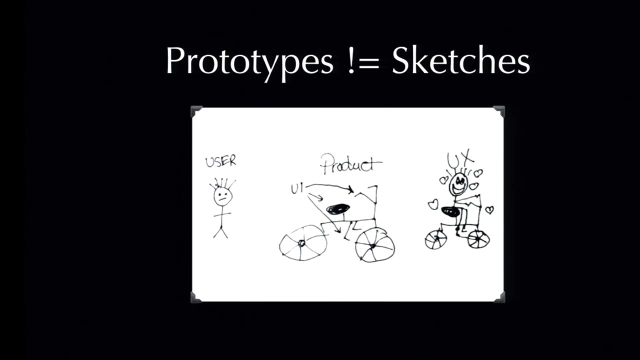 testing, which is the most important part. First of all, what is and what isn't a prototype? Well, prototypes aren't sketches. Sketches are freehand drawings that we can quickly and easily make to visualize ideas and communicate with others. It is in no way meant to be a model of the 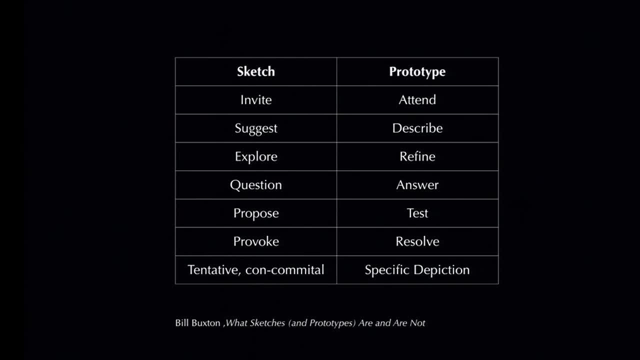 final website. According to Bill Buxton, who's the principal researcher at Microsoft Research, who's also known for being one of the pioneers in human-computer interaction design, he thinks the difference between sketch and a prototype is the following: Sketch is used to explore ideas, It's used 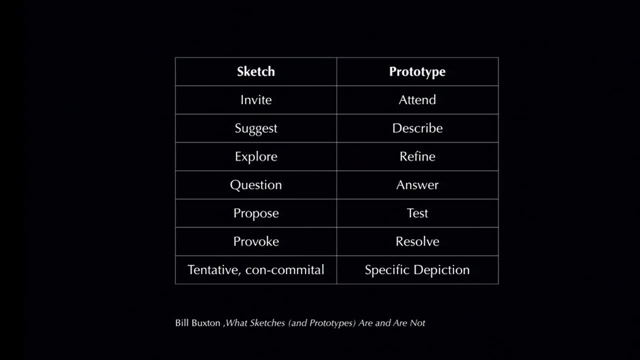 to raise a question, to propose a potential solution, to make suggestions, to invite people to come and collaborate with you, While prototypes is to describe a solution to refine and test your design, to answer questions and to test, especially usability testing. Secondly, prototypes: 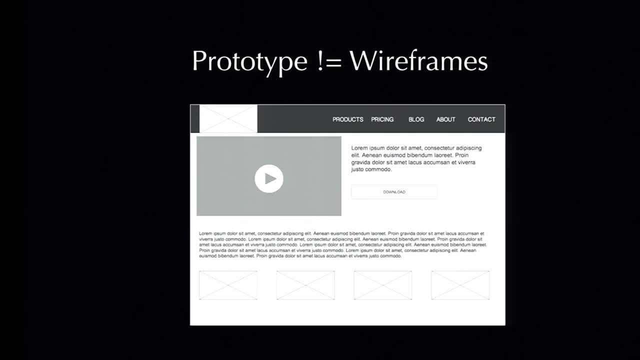 are not wireframes. Wireframes are visual layout of a website. It doesn't include any functionality of the website. It doesn't have animations. It doesn't have clickable navigations. It doesn't have change of page state. It tells you where each component of the page will leave. It gives 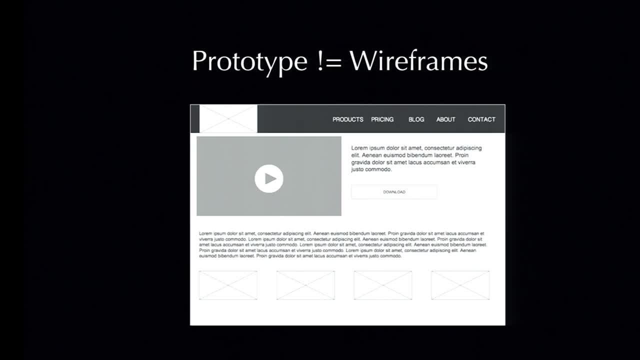 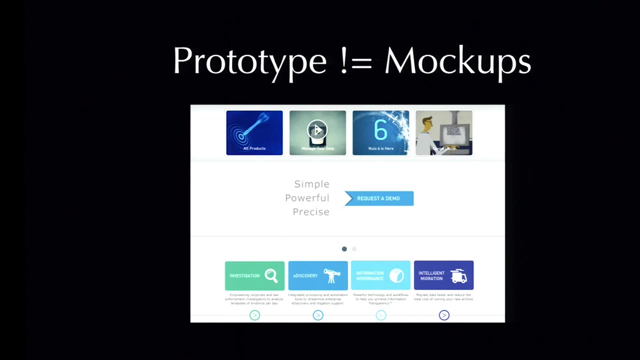 you some insight into the site map hierarchy. However, now as wireframes become interactive- I mean, when I click on the menu, it will take me to another page- Then these wireframes become a prototype. Finally, prototypes are not mockups. Mockups are visual design of a website. It doesn't. 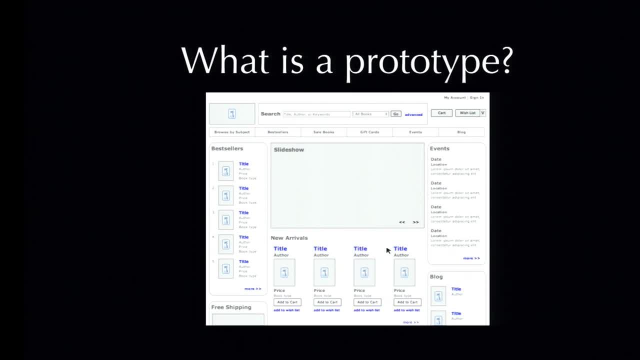 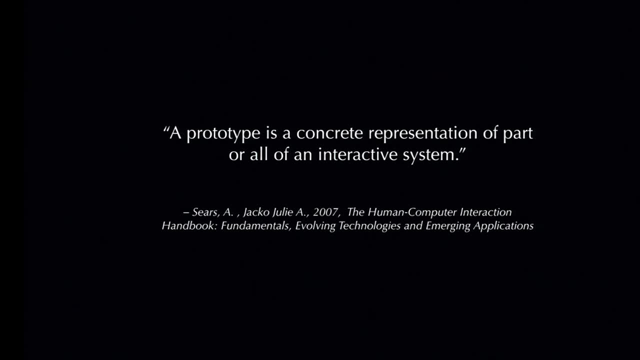 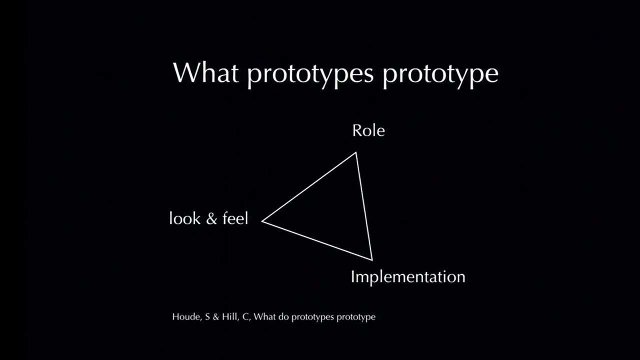 include any functionality of the website. Now, what is a prototype? According to the Human-Computer Interaction Handbook, a prototype is a concrete representation of a human-computer interaction. It's a representation of a part or all of an interactive system. What does that mean? Well, interactive. 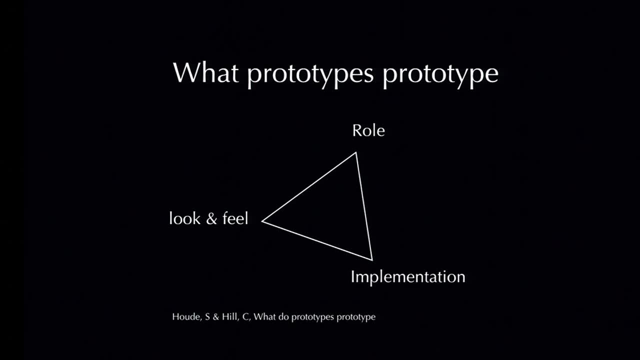 systems have three important aspects. The first is the role, which means what role does this website play in the user's life, In which way it is useful to them. For example, with PayPal, you pay someone. Implementation means the functionality of through which component and techniques this website. 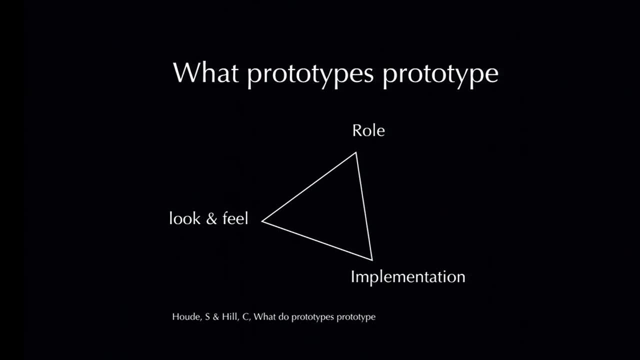 implements its functionality. So what is a prototype? What is a prototype? What is a prototype? What is an interactive functionality, For example, for a Drupal site? we use Drupal, We use PHP, We use HTML JavaScript. Look and feel refers to concrete sensory experience a user has when they're using the 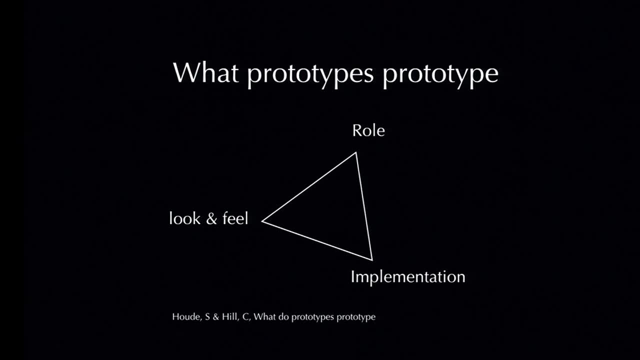 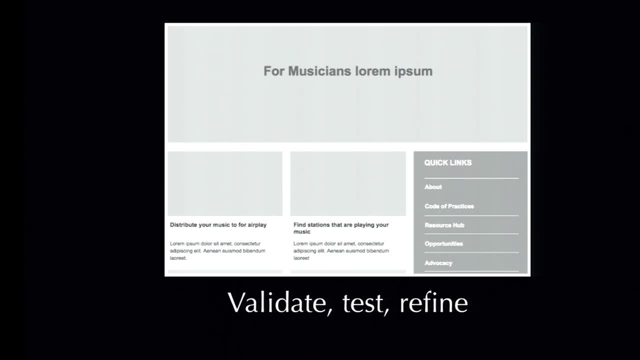 prototype. Why do we need a prototype? First of all, prototype is to validate, test and refine our design. It has to tell us what works and what doesn't, before we even start building the site and writing custom modules. It gives developers, designers. 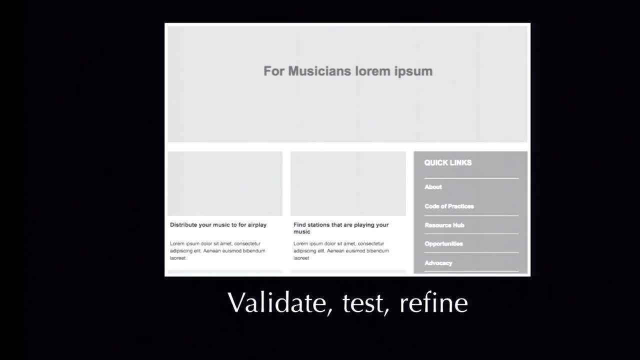 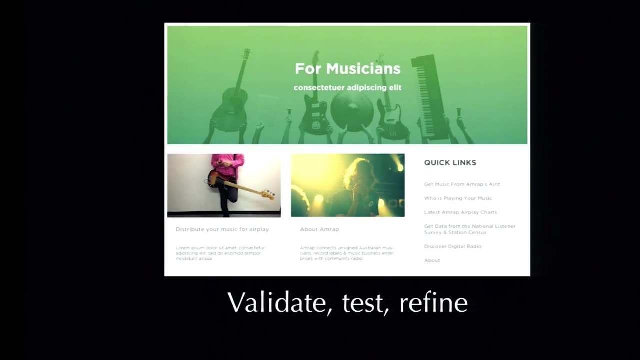 and project managers the confidence that whatever they're going to do is going to work based on testing. So once you have a prototype which has been thoroughly tested, The site builders can just go in and start building the site And the final design won't differ much. 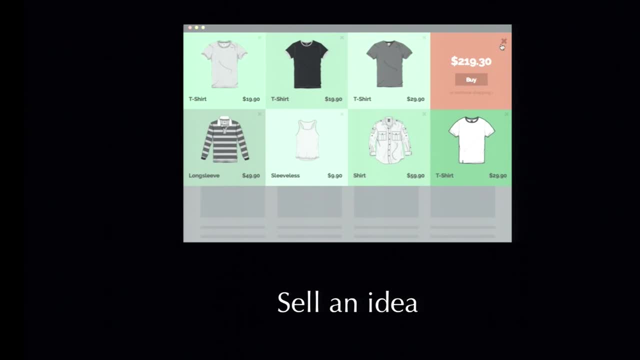 The second reason we need a prototype is we can use it to sell the idea. It's always easier to pitch to a client if you have a concrete prototype for them to test on and play with, rather than just trying to tell them in words what 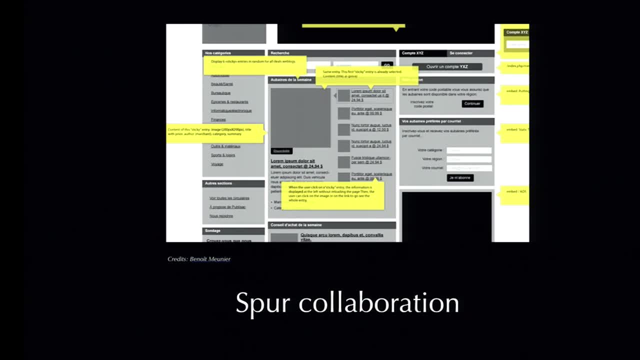 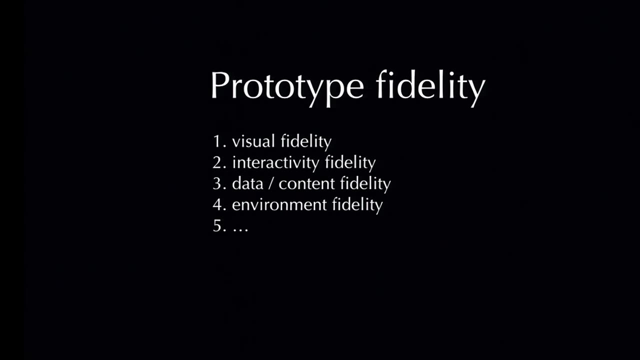 you are trying to do. And thirdly, prototype is a great way to spur collaboration. Clients, developers, designers- they can all come together, work on one prototype feedback directly into the prototype. So now it comes to prototype fidelity. When it comes to fidelity, we talk about low fidelity high. 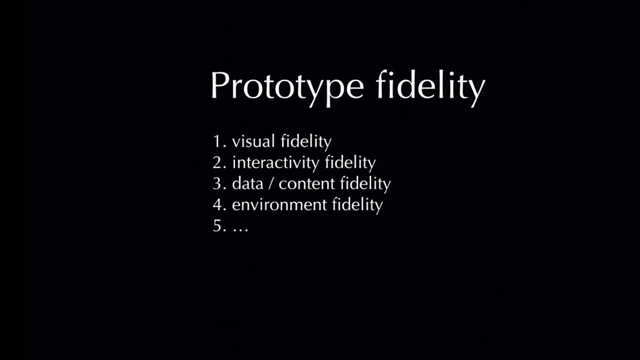 fidelity, But it's actually just one aspect of prototype fidelity. We have many levels of fidelity in prototype. We have visual fidelity, which means how polished this prototype is. Does it look like the final website? Interactive fidelity: Does the prototype have the same animation and translation? 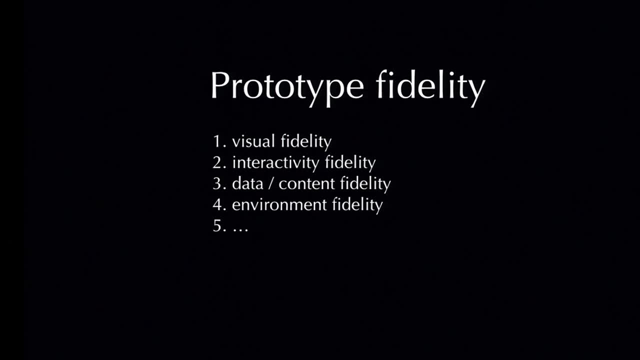 with the final website? Data content fidelity: Does the prototype have the real data and content And environment fidelity? Does the prototype work on mobile? Does it work on tablet? How does it work at home, at work in different browsers? That's environment fidelity. 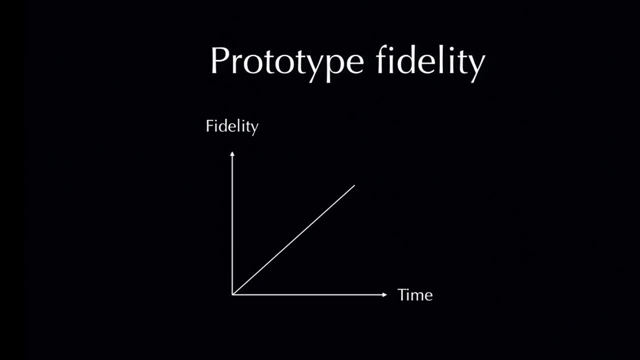 And there are many other aspects of fidelity. I'm not going to bore you with the details here, but you can see it. However, with the increasing fidelity is the increase of time and money. So in the world of prototyping it's not always the more the 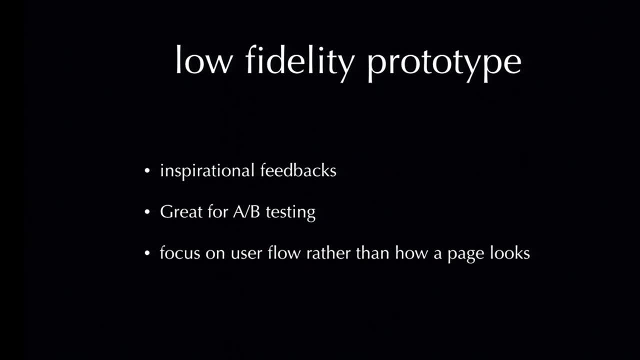 better For most projects. for some projects, especially most projects in agile development, will have several version of prototype, iterating from low fidelity to high fidelity. However, in some projects that doesn't have big budget, it's always good enough to start from low fidelity prototype. 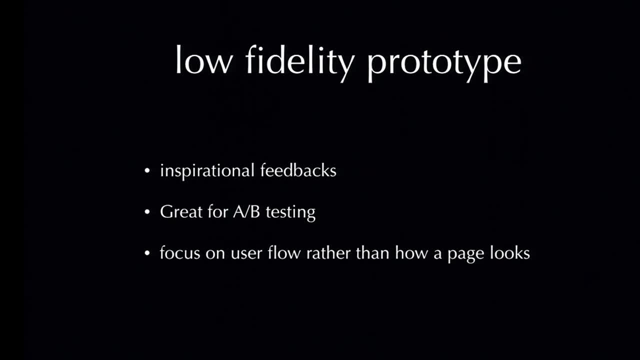 It's cheap, It's easy to make. It gives very inspirational feedback to the designers, because testers don't have to worry about building onto the designer's idea, They don't have to worry about the design. They don't have to worry about the design. 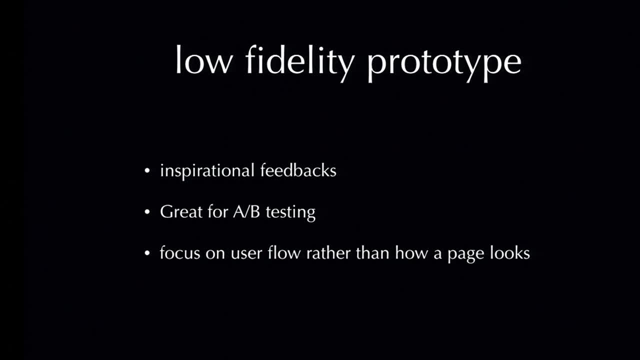 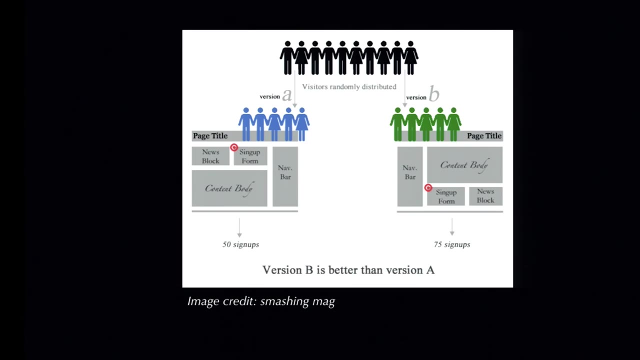 They don't have to worry about upsetting the designers. They can just say whatever they want to say. Secondly, low fidelity prototype is great for A-B testing. So do everyone know what is A-B testing? So a quick explanation. A-B testing is a usability test that we create two versions of. 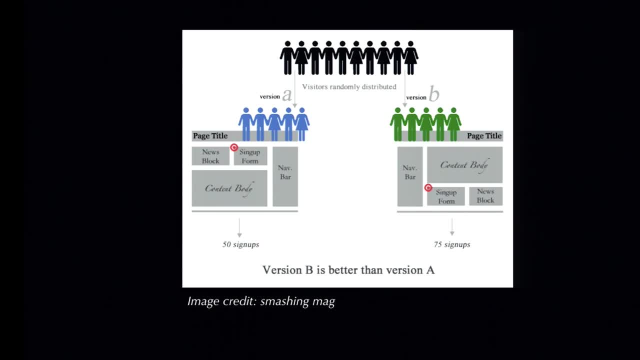 UI element and we set a matrix for success. For example, here we have: on version A, we have signup form on the left, on the left of the nav bar, behind the page title. On version B, we have signup form behind the content body on: 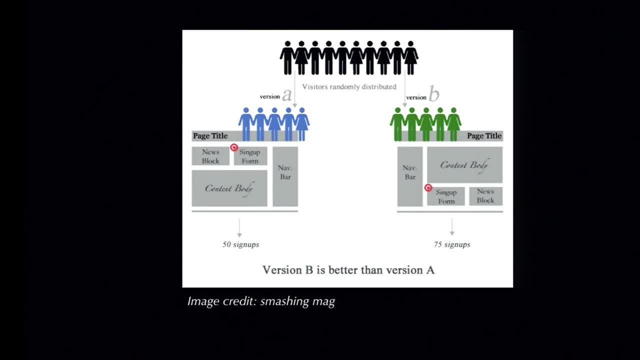 the right-hand side of the nav bar. Then we have two randomly distributed user to test on both prototype. In version A we have 50 signups. In version B we have 75. That means version B is more effective than version A. 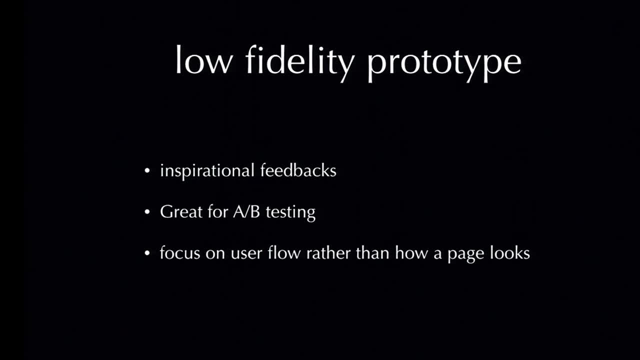 So in low fidelity prototype, A-B testing is easy because it's easy, quick and cheap to move around the UI element. Thirdly, low fidelity prototype allow testers and designers to focus on user flow and the task flow rather than being distracted by colors, typographies and images. 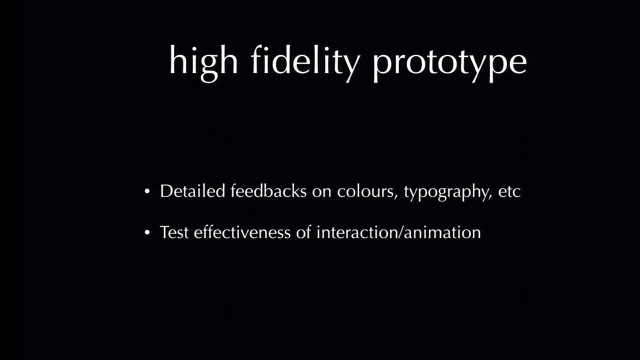 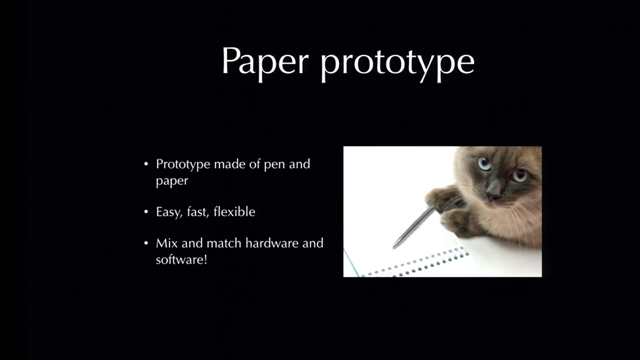 However, there are times when we need to use high fidelity prototypes. That's when we need detailed feedbacks on colors and typographies And so on, Or we're trying to test the effectiveness of animation transitions. So different type of prototypes- Paper prototype- by far the most common one and the most 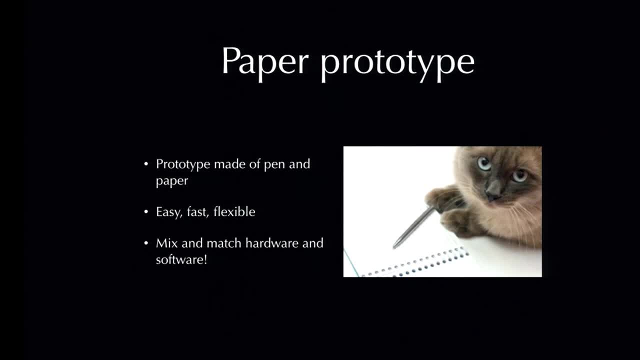 easy to make one: No learning curve, Everyone can sketch, And there are softwares nowadays that allow you to upload your drawings into the computer and build interactions based on that. I have here a quick case. This is a quick example paper prototype I created. 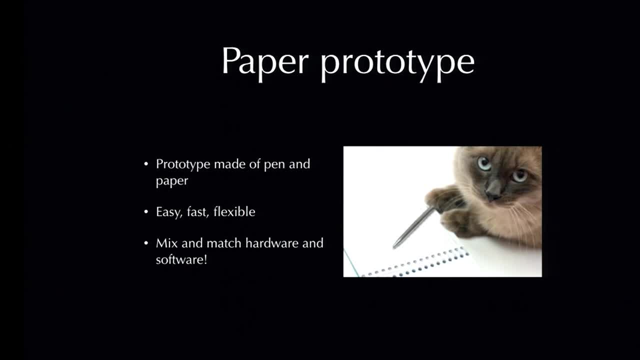 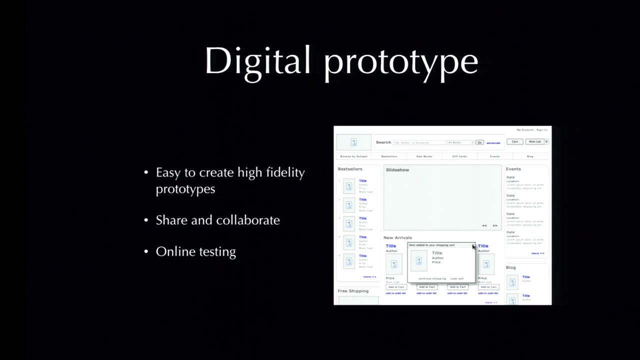 So if you're interested, you can come to me afterwards and I can show you how it works. So, basically, we use post-it or paper to indicate page overlays and markers to indicate UI element And, of course, we have digital prototype. Digital prototype: it helps us to easily create high fidelity. 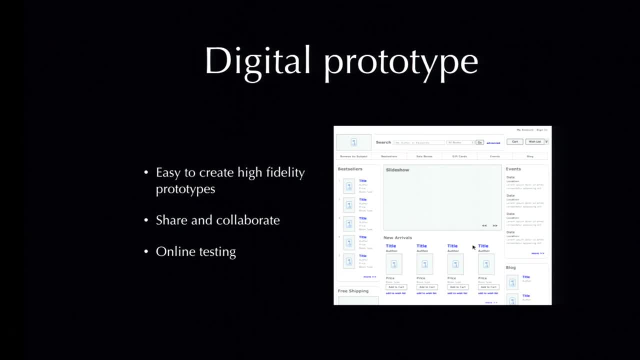 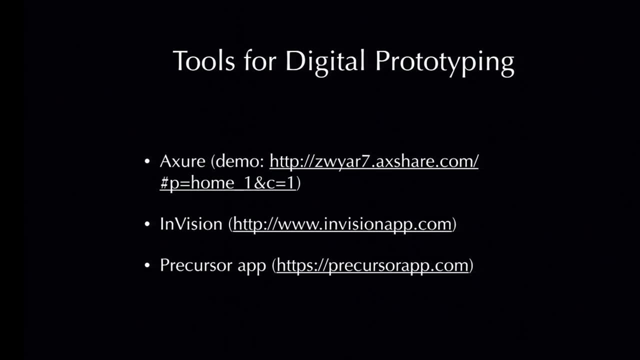 prototypes. So I hope that's helpful. Thank you, Bye bye. It's very easy to share and collaborate with others. Once you put it on a server, everyone has access to it, And it's great for organized online testing. I'm going to briefly talk about some tools I use for digital prototyping. 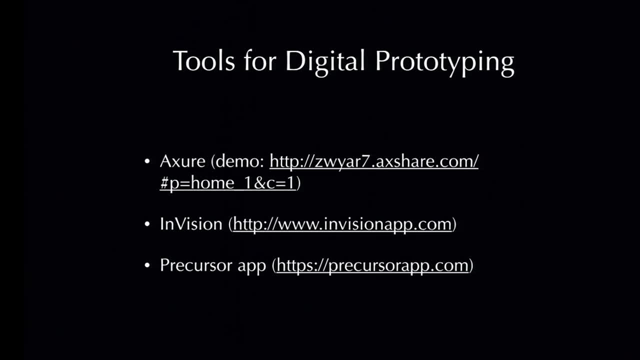 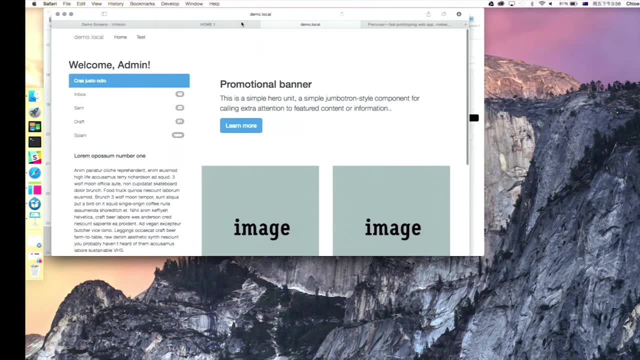 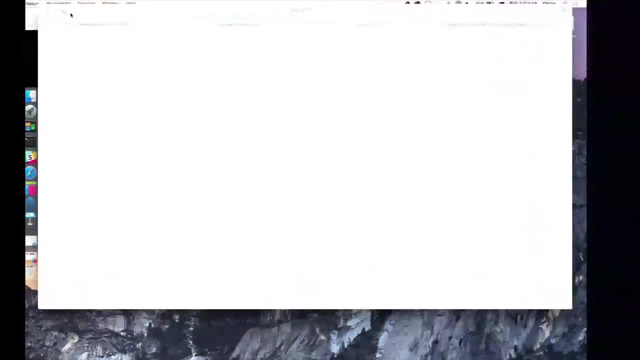 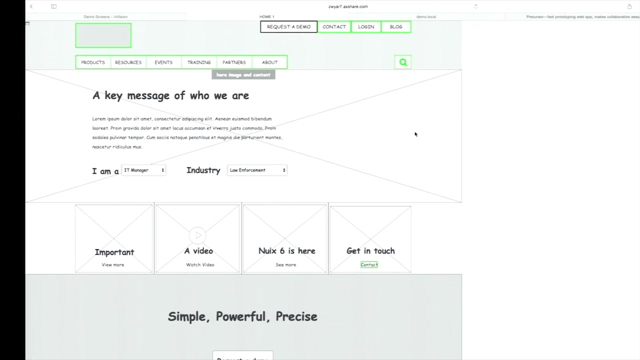 The first one is actually. I'll show you a demo Here. we go, Bear with me for a second. So here is a digital prototype we have created earlier for a client using Action. As you can see, we can have different page menus. 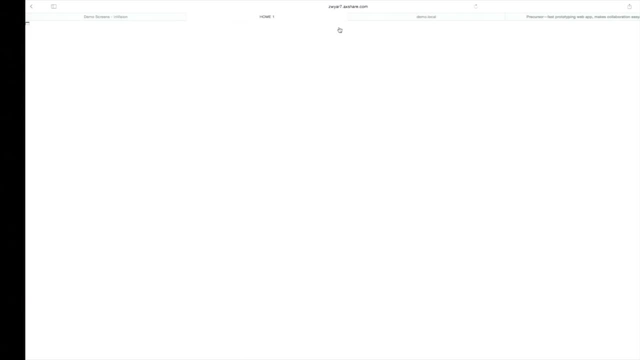 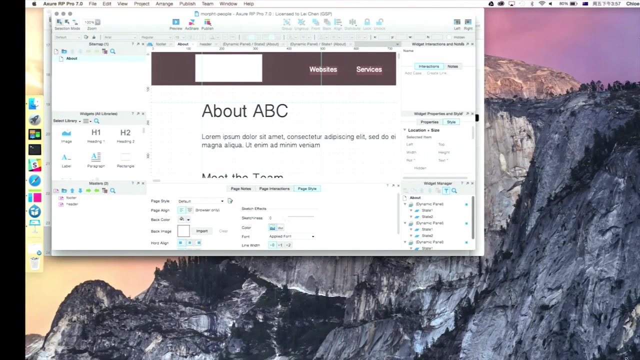 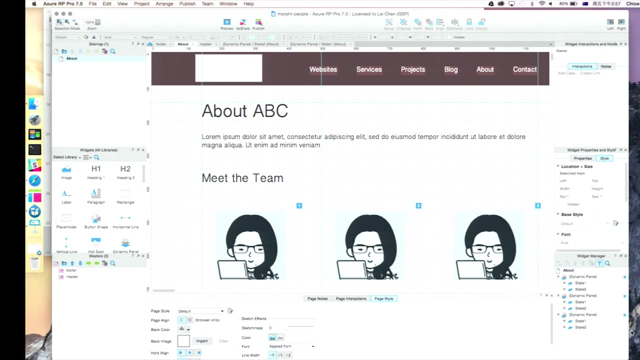 dropdowns, select box, We can go to different pages. It's very slow. We can have web forms, maps and so on. It's very easy to create high interactivity fidelity prototypes in Action, Just to show you that I'm not lying about it. 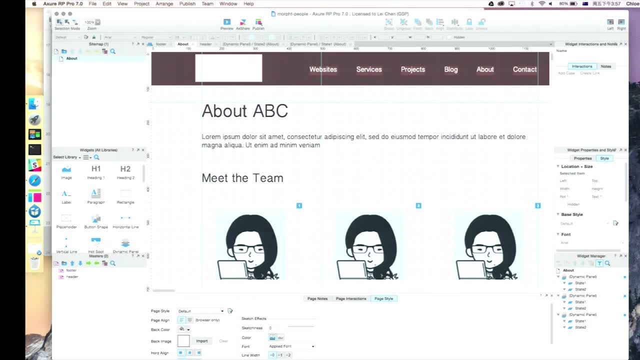 I'm going to quickly create one. So this one is I created earlier. It's about page. This is the user interface of Action. So I'm going to create a new page. So I just click here: A new page. 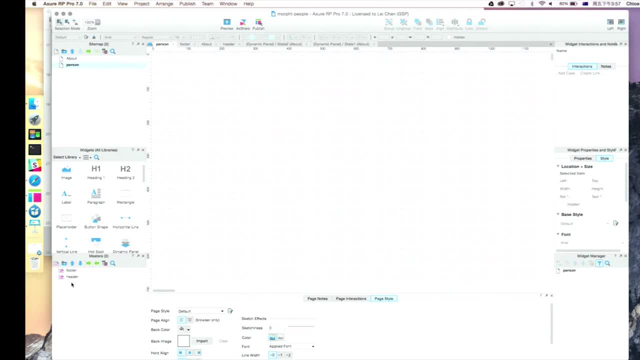 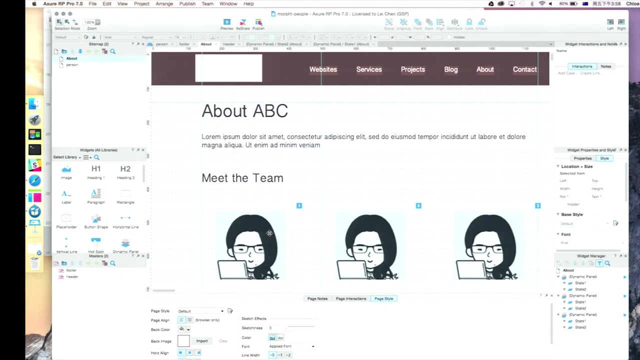 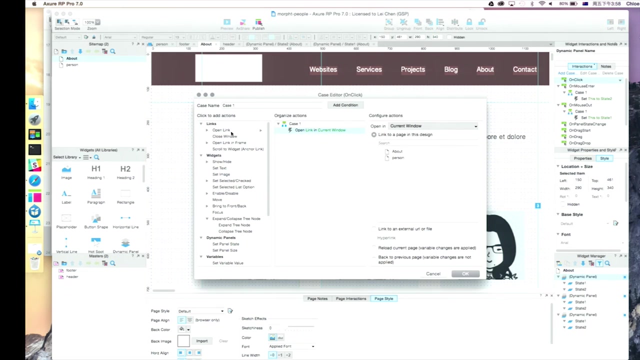 Call it person page And then come here. I have predefined header and footer so I don't have to do it The second Time. Heading here, Image: A very ugly page. Now I want to create some interaction. I want to happen that when I click on this it goes to the next page. 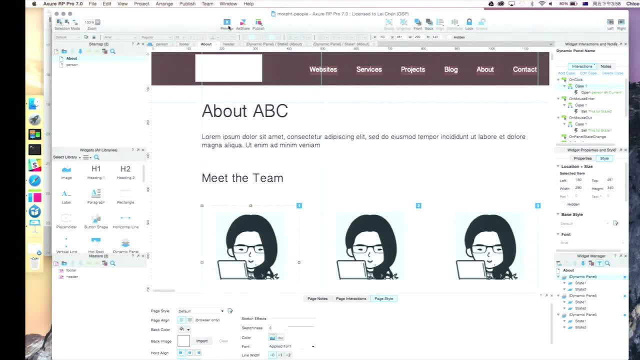 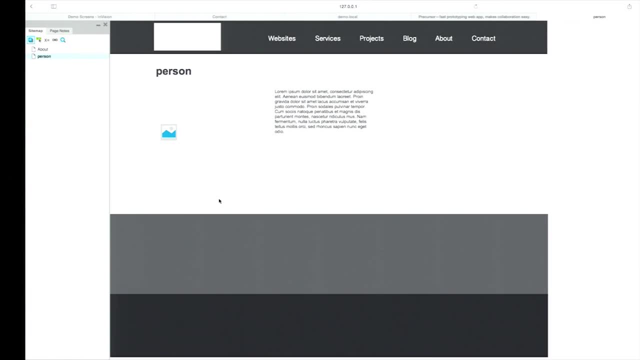 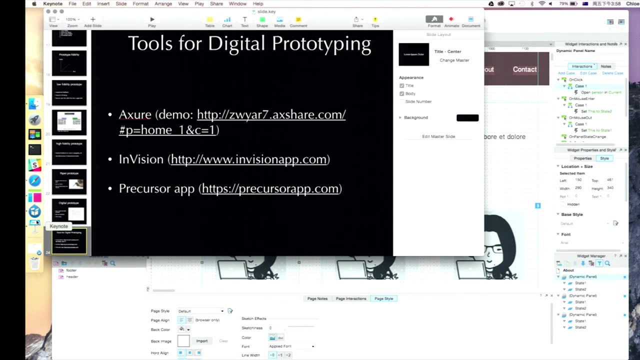 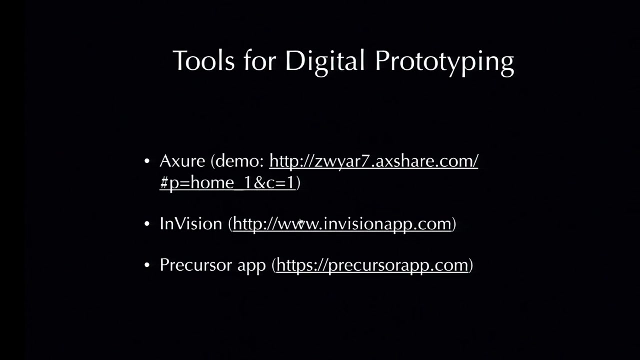 So I create on Click Invent, Open link, click open to person page and now I preview it. When I click on it it goes to my very ugly page. That's it. It's that easy. The second tool I like to use is InVision, The 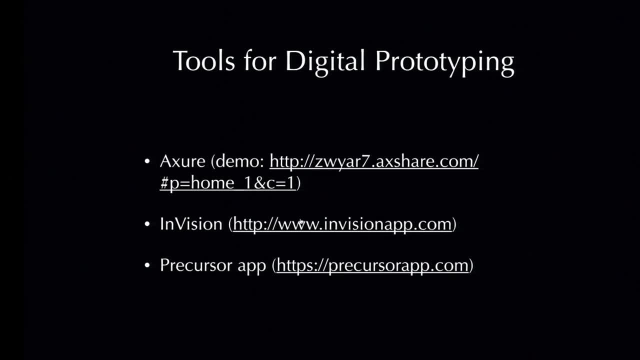 difference between InVision and Acture is you create your element in Acture by yourself. It's very easy to do high interactivity prototypes Well in InVision. you upload your designs into InVision and build interaction based on that. It means you can have fabulous high 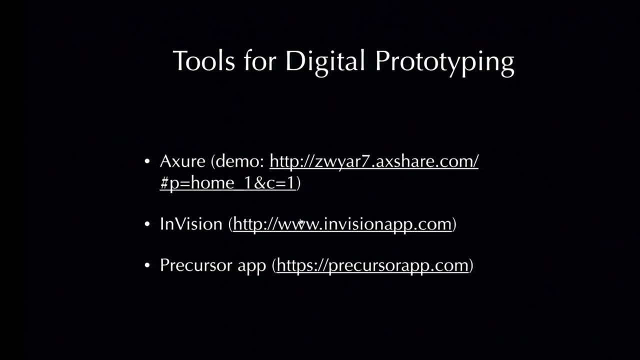 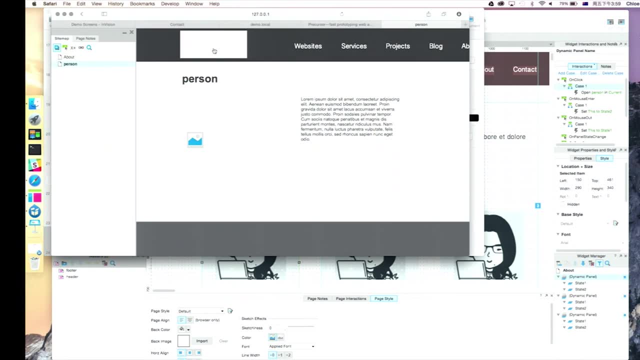 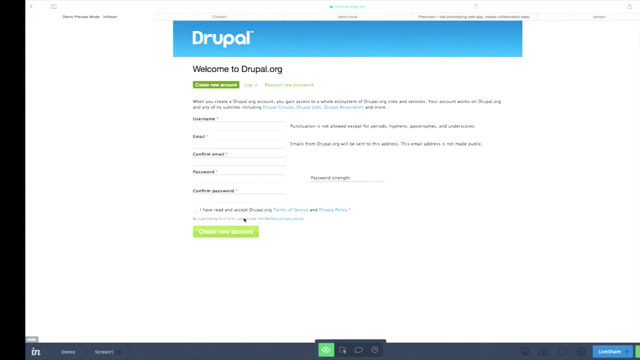 visual fidelity prototypes that look exactly like your design And you can create very basic interactions. I have an example here, So here's an example I created earlier using Drupalorg. What I did was I just took a screenshot of Drupalorg sign-up screen and did a bit of upload to InVision and added a bit of interaction. 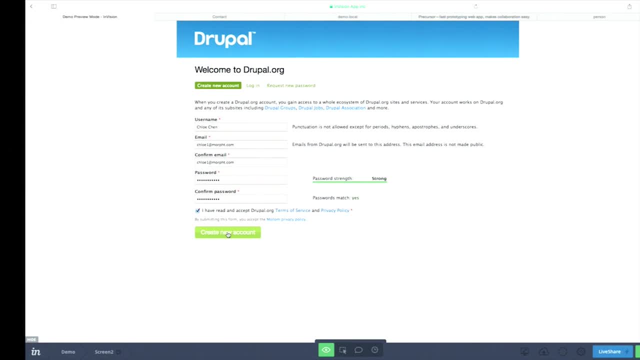 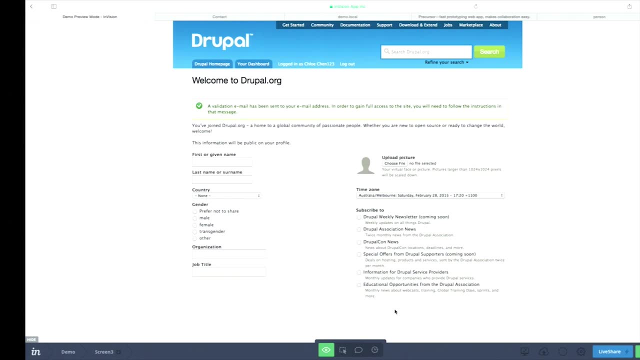 As you can see, it's very easy to do high interactivity prototypes. It's very easy to do high interactivity prototypes. If I click on the username field, it fills up for me And I click create new account and it goes on and creates a new account. It's a very good tool to show to. 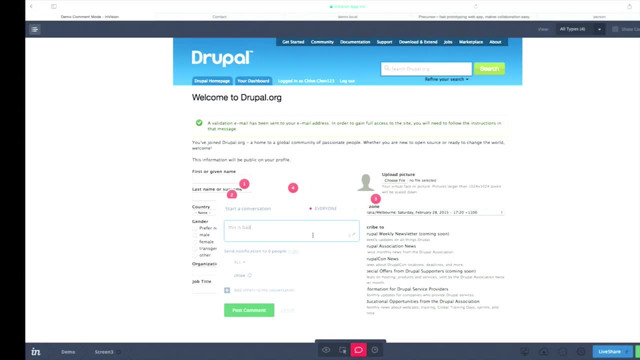 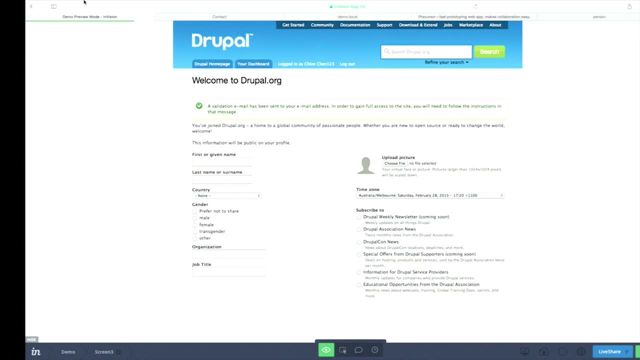 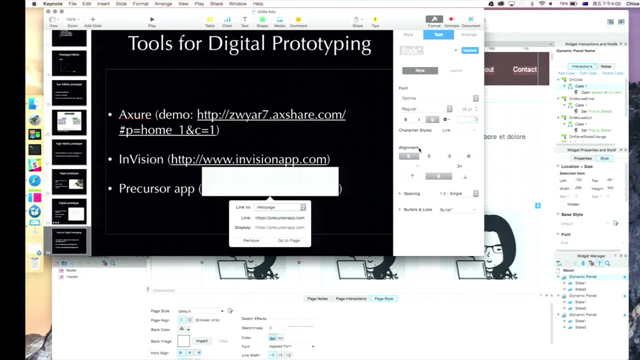 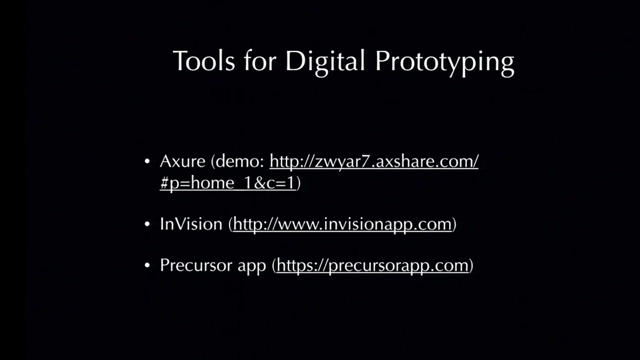 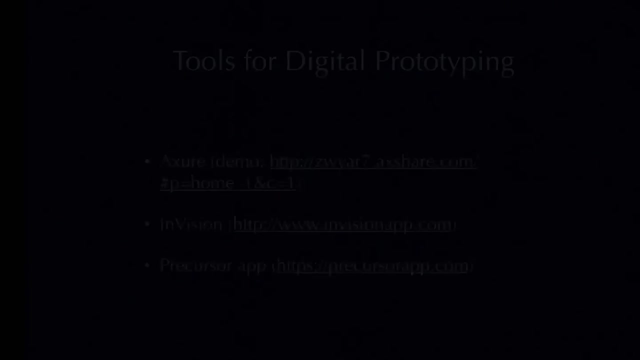 clients because they can just go to common mode and say something like this is bad. I don't know how to get out of this. And the third tool I just discovered a few weeks ago is called Precursor. I love the simplicity of it. Compared with Axure and InVision, it's just so simple and it works. 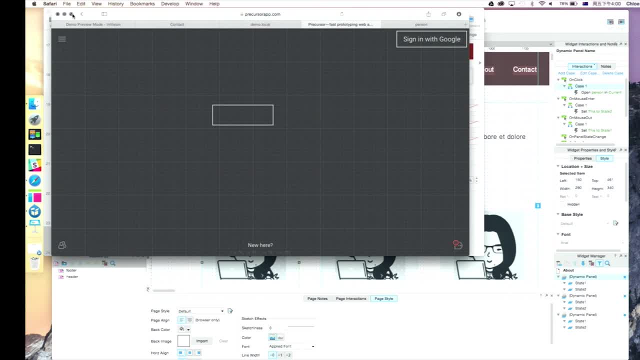 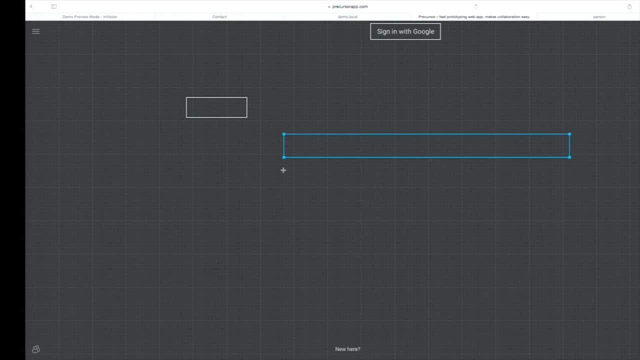 on tablet. A quick example as well. So you have only five tools, but you can quickly put on your ideas and some text and share with whoever you want to share. It works on tablet, so it means you can actually draw with your hand. 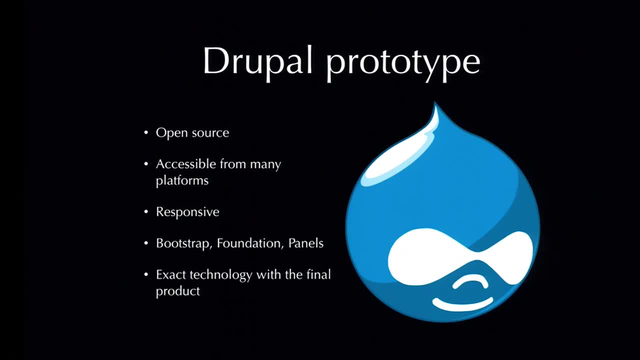 So here are digital prototyping tools And, of course, for all of us here, we can do prototyping in Drupal. Well, Drupal is open source, It's free and for all of us here there's not much to learn. And with the thing with digital prototyping and paper prototyping is that 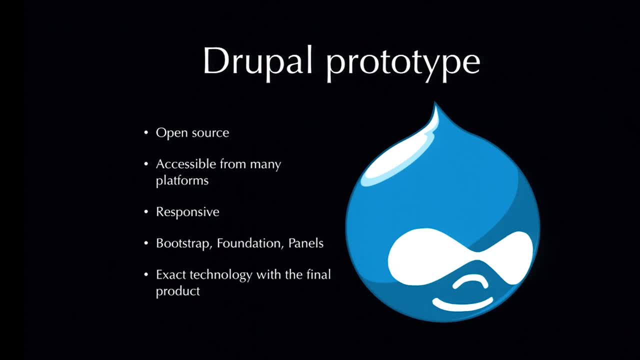 if you want to do a prototype that works on mobile and tablet and different devices, you need to create at least three of them. In Drupal, you create one And by using a responsive framework, it works everywhere, especially with the framework such as bootstrap foundation. 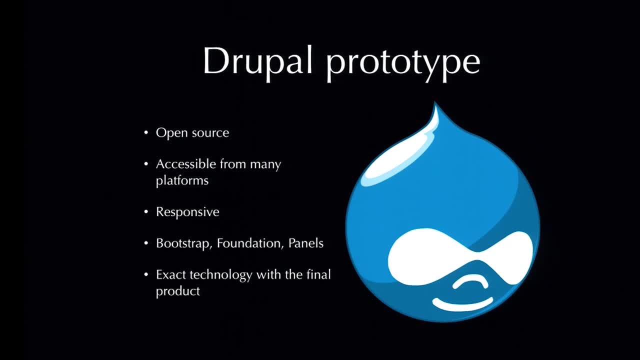 and modules like panels and display suit. It makes Drupal prototyping really easy. The advantage of Drupal prototyping is that you're using the exact technology with your final website. This is especially good for agile development When you have a version of prototyping and 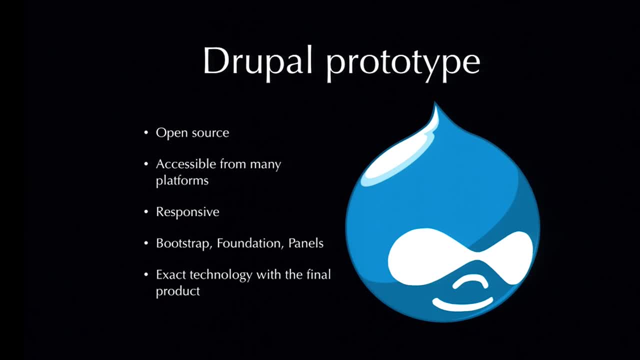 you test it. by the end of this sprint, the designers get all the feedbacks from stakeholders and users and then put it into the next iteration Until the final stage of the project. your final prototypes become your website- Another situation when Drupal prototyping can be useful. 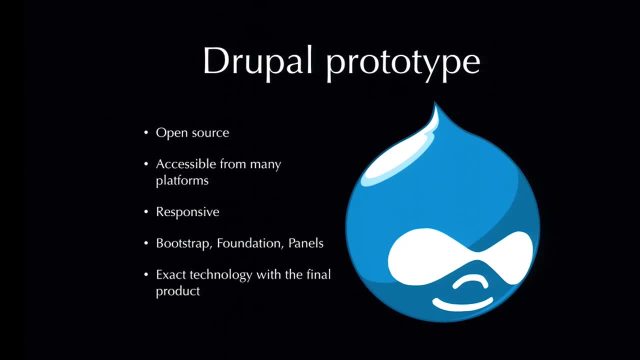 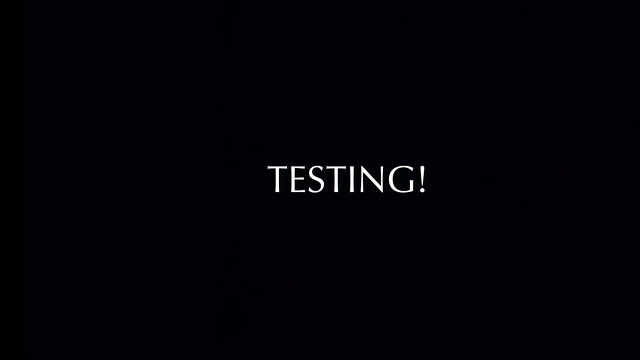 is, in my opinion, when you are creating one or two new designs for an existing website, You already have all the nuts and bolts for the website. You have the views, you have the content types, You just prototyping Drupal, get feedback, iterate and then that's it. 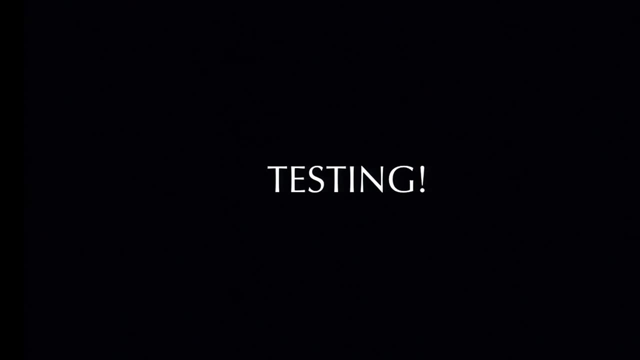 So now we have prototype and we come to the most important part, which is testing User-centred design. User feedback are the most important source of feedbacks And the prototype allows us to put user testing at the beginning of the project rather than at the end of the project. 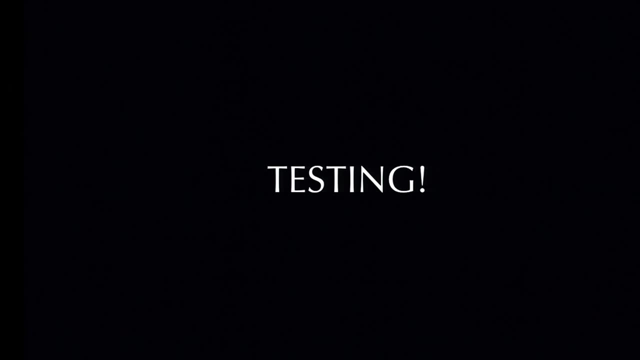 So, as designers, we shouldn't make any assumption that what works and what doesn't. All the conclusions should be drawn from testing. In the ideal world of testing, we have real users sitting in front of us: Stakeholders, high-profile users. We have a lot of users. 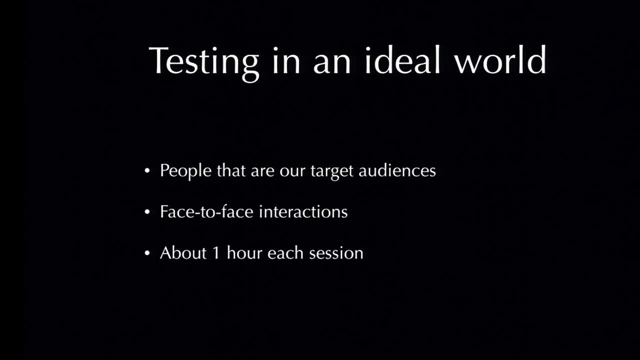 hiding behind some one-way glasses looking at us. We spend about one hour each session with a user. We do at least five users a week. However, this is not always possible, And then online testing come to rescue. I'm going to talk about a few types of online testing here. The first one is usability hub. 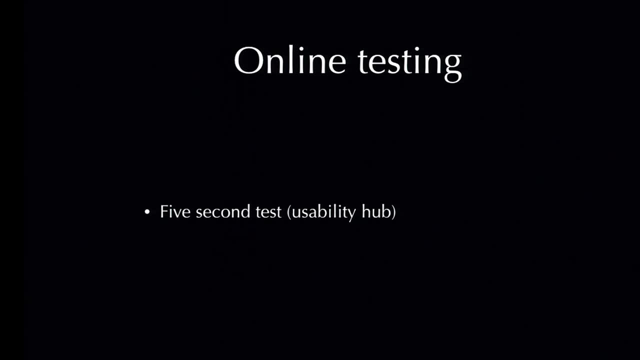 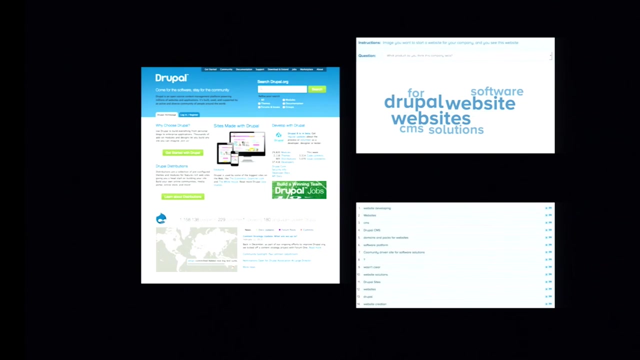 Offers this. The second one is five-second test. Five-second test is based on the principle that users only look at your design for five seconds And if you fail to impress them, if you fail to make them take action, then you fail. So here's an example, again using Drupalorg. 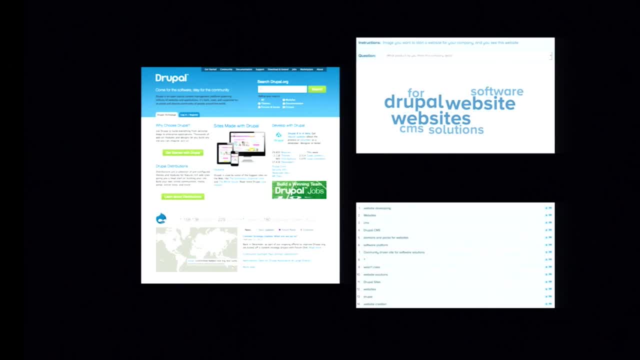 What it does is it lets users look at a screen for five seconds only and ask them to answer a series of questions. Here I use Drupalorg home page. Let users look at it for five seconds and ask them: what do you think this company does? I get a report of the answers And then from the report 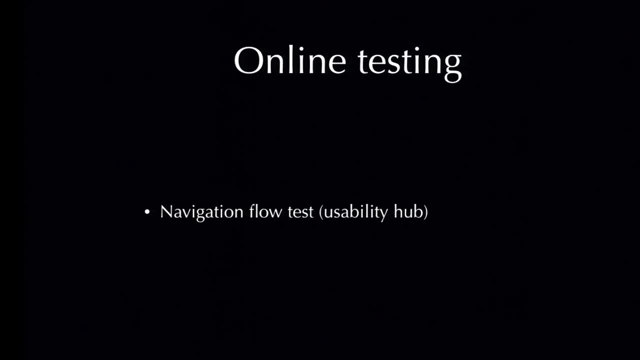 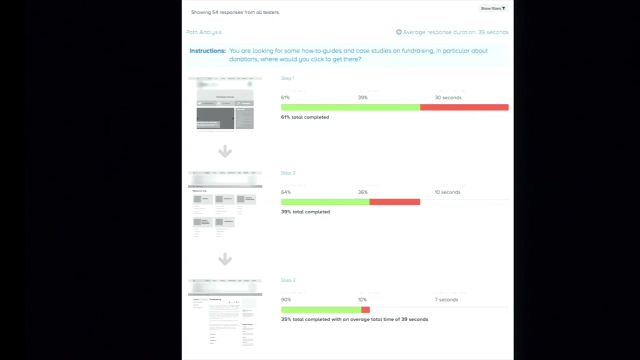 I can see whether my key branding is getting through to the users. The second type of test is navigation flow test. It works by letting users complete a task by going through your navigation system. Here's an example. I have a less user to try. 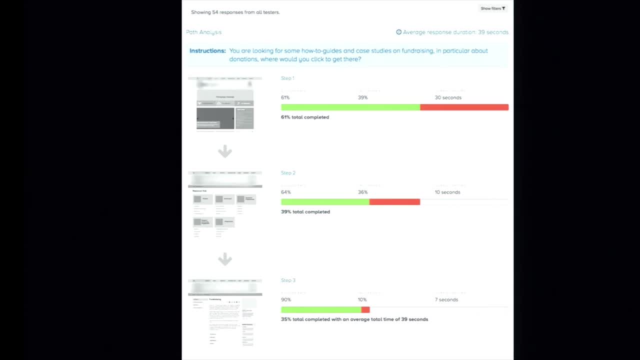 to find out a piece of content on my prototype. As you can see at each stage, some people managed to do it, Some people dropped off And this report show me the average response time. This is great for testing whether you have a client. 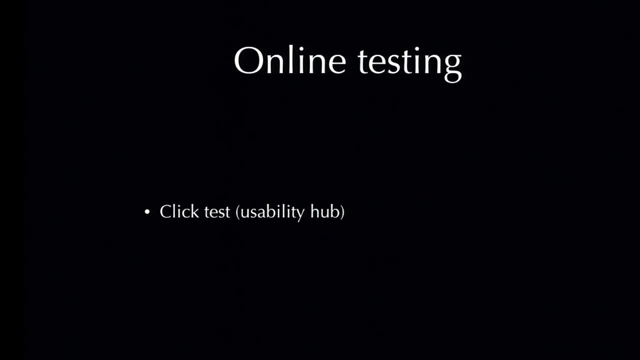 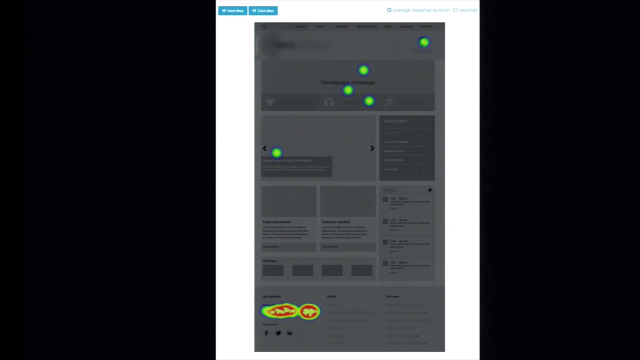 clear, understandable navigation system. The third one is click test. Click test can be used to test your call to action buttons or newsletter sign up. Example: here I have this prototype. I have the newsletter sign up here. Oh, what's happening? 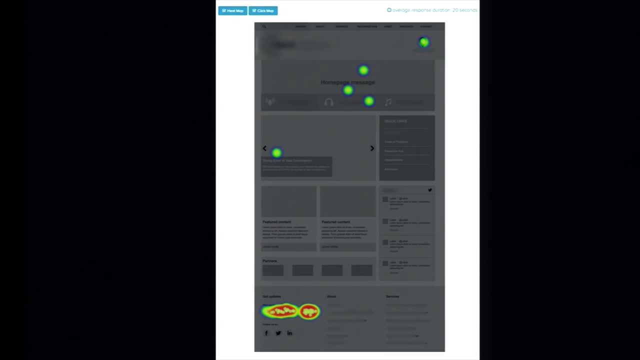 I'm sure I didn't do it And ignore it as if it's not there. So, yeah, my prototype is too awesome. It's good. So, yeah, I have this newsletter sign up button here And, of course, it's a very successful one. 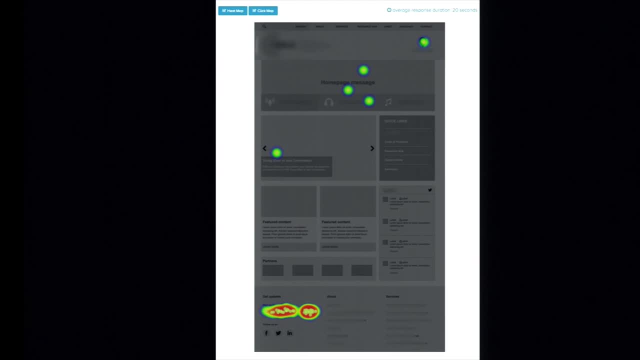 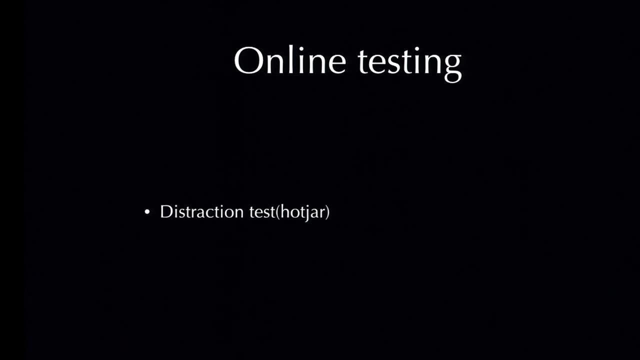 Only a few clicks as well, But by doing this type of test you can see whether your call to action is working or not. And the last one is distraction test. This is used to test whether the key message on your web page is prominent enough or whether your page is too. 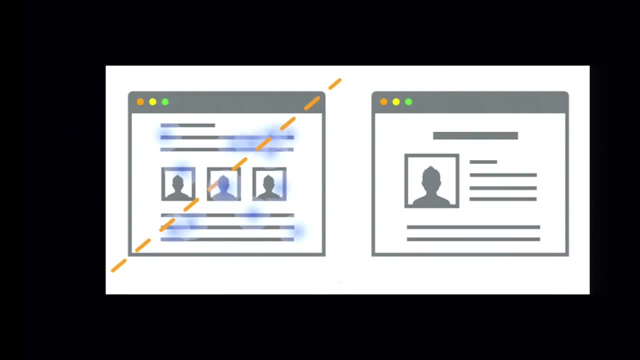 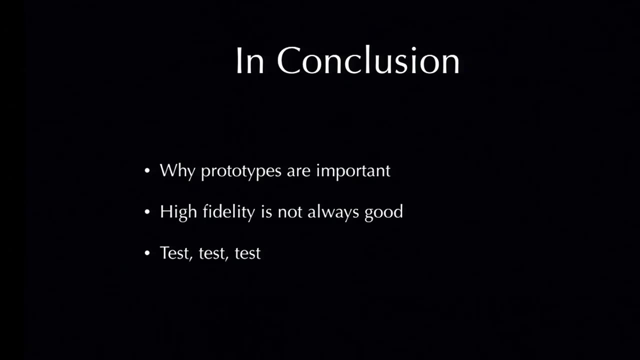 cluttered or too busy for people to really see what you're trying to see. So here's an example. On the left, we see users basically clicking all over the place. That means the page is either too busy or the key message is not prominent enough. 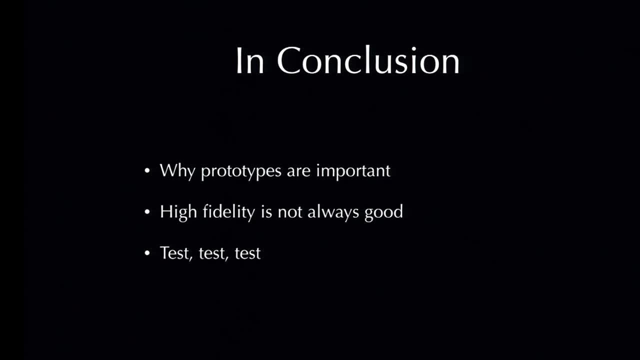 Well, in conclusion, prototypes are important. It is one of the most important deliverables in UX design. And you might say what, if I don't want the whole full-on UX design process, I want Lean UX. Well, prototype is in Lean UX prototypes. 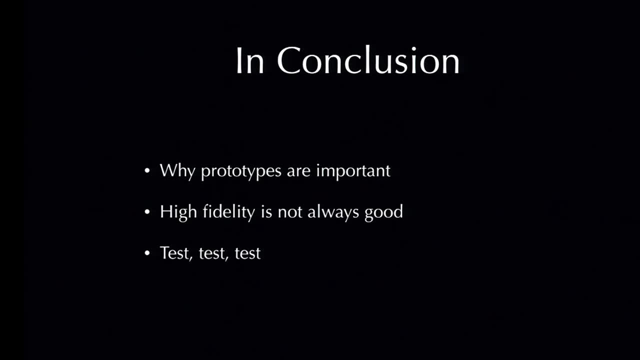 shine even brighter because it helps you to avoid the most obvious mistakes. Just do a low-fidelity prototype. Keep your focus on the key element and you can avoid making heavy, costly mistakes in later stages. Again. low-fidelity prototypes sometimes are more effective. 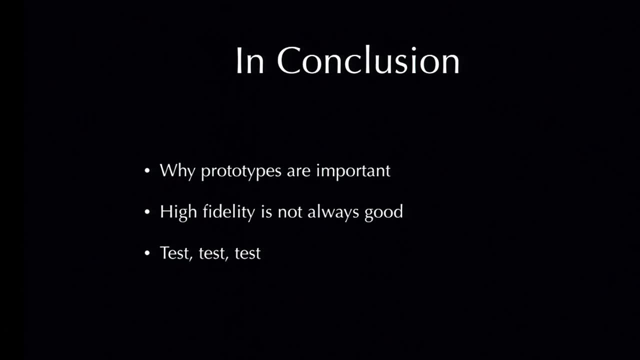 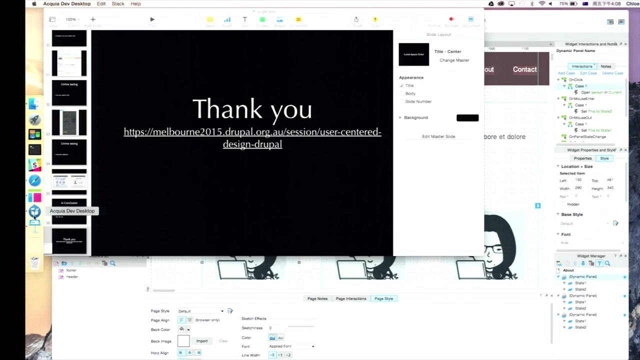 than high-fidelity ones. And the most important thing is we do usability testing thoroughly. Don't make any assumptions. Thank you, That's all Any questions? Do you have any Bootstrap-specific tools that you like to use for prototypes? Yes, 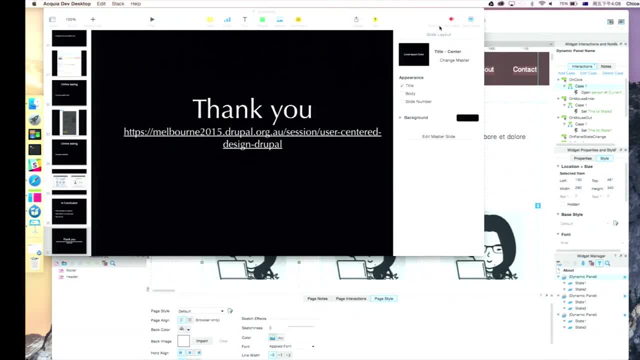 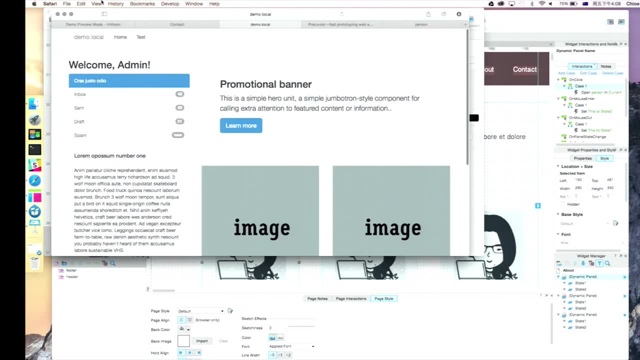 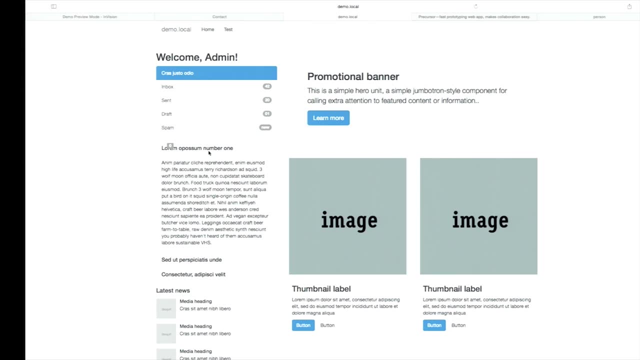 OK, So I use Bootstrap when I'm creating a prototype in Drupal. I have an example here. So this prototype is created in Drupal. I used the Bootstrap theme and the panels. No single line of code was written, And then you already can have all the things. 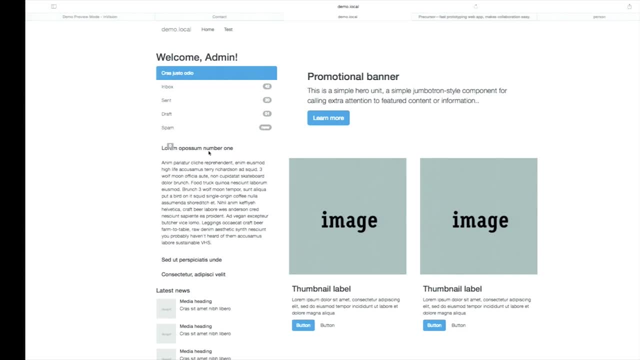 It's all sort of layout. So yeah, I hope that answers your question. I have one suggestion. Have you heard of the Pencil Project? It's an open-source alternative to Actuva. No, I haven't. I can recommend it. 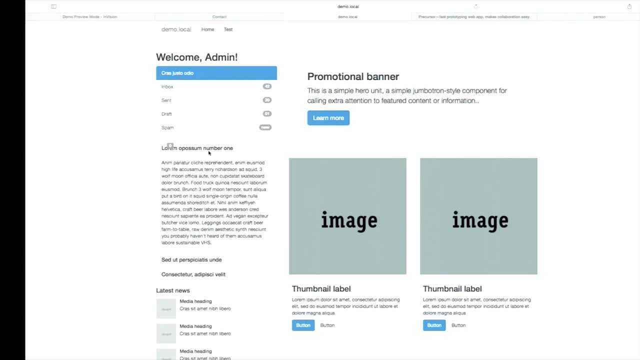 It's free, It works very, very easily. Yeah, I'll definitely have a try. What was it called? again, The Pencil Project? OK, Have you worked with Foundation doing the same thing as this? Yes, It's more the power of panels that gives you. 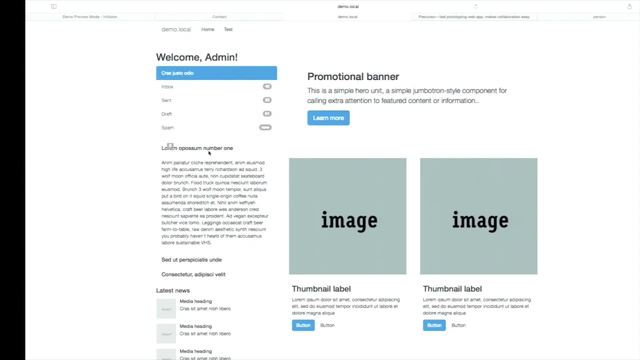 that really good prototyping thing, is it? This one? it's more power panels that deal with the layout And Bootstrap that deal with, for example, the media object, the thumbnail, what is called accordion stuff. Yeah, definitely, Foundation.